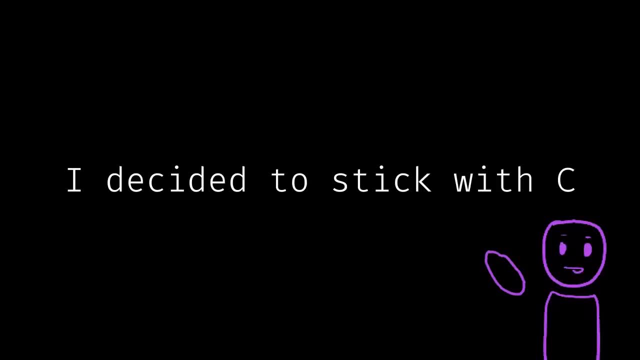 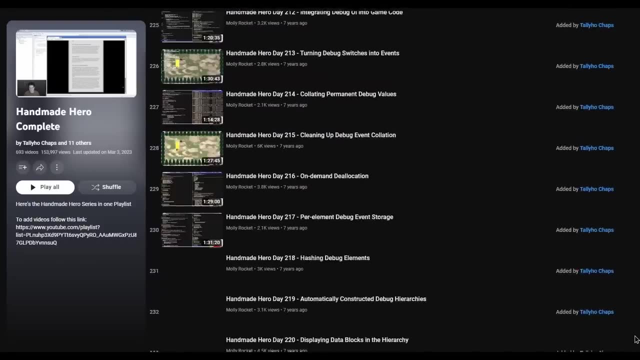 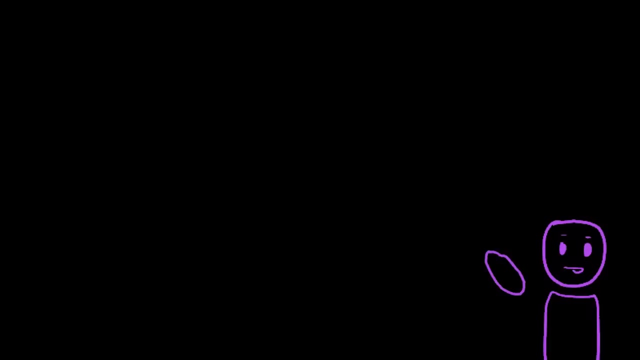 the sake of my curiosity, I decided to stick with C for the time being. That's when I discovered the wonderful handmade network and found a massive obelisk of knowledge that is handmade hero and dug deeper and deeper into low-level software development. I looked into libraries like 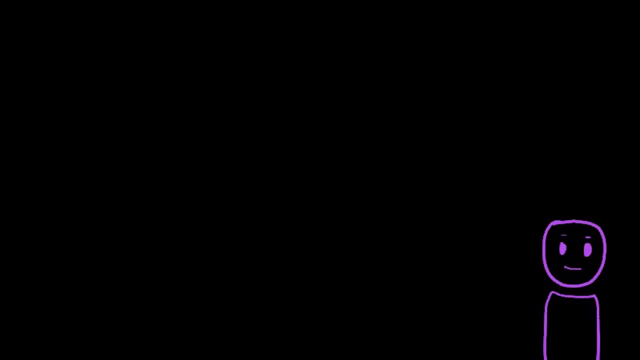 Raylib and Gunslinger to figure out how graphics programming was done. I already knew a bit of OpenGL, since I came from Java, but figuring everything out in C was incredibly fun. After about five months, I felt I was ready for my first project Circling around to the reason. 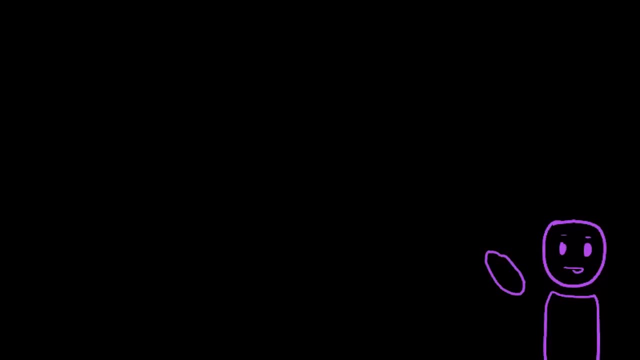 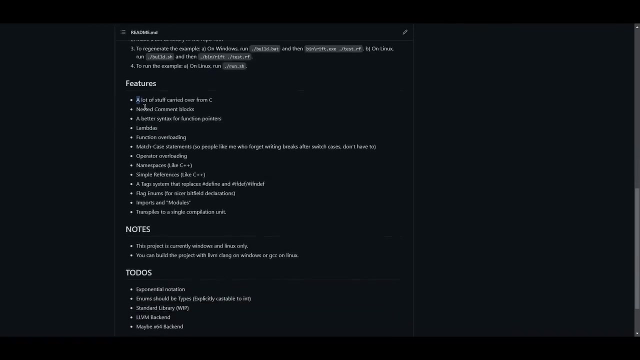 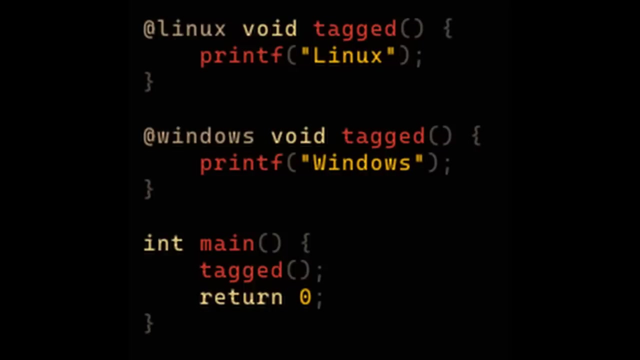 I came to C, I decided to write a programming language transpiler. I got really far too. It had all the basics from C implemented and also some things from C++ that I thought were nice, like function and operate, overloads and references. I also had a completely new system for tagging. 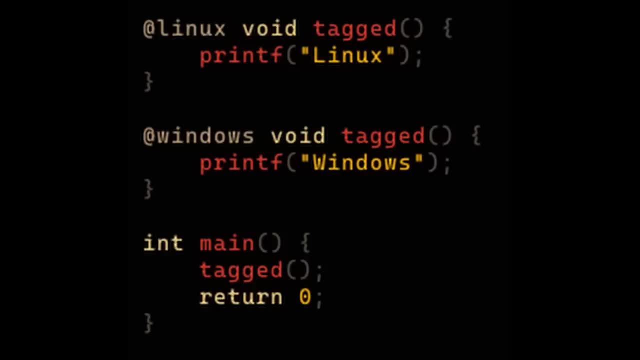 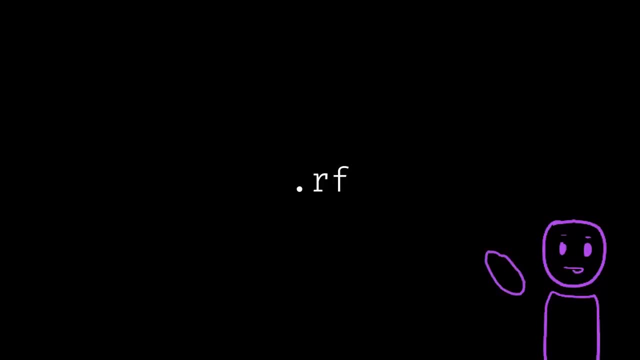 statements which acted just like the hashtag- if they're preprocessors statements, but with a nicer syntax. But then something hit me. I'd been transpiling everything to C code, but this made step debugging pretty much impossible, since C compilers would emit code with debug symbols based on the transpiled code and not my own. So I tried working on an. 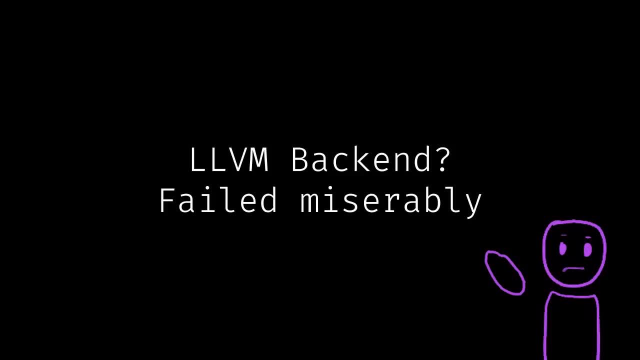 LNVM backend, but quickly ran into some weird issue when trying to add Linux support and gave up. I still had learned a lot by working on the project, though, so it wasn't a complete waste of time. I found out that many of the memes seen online about C's unsafety 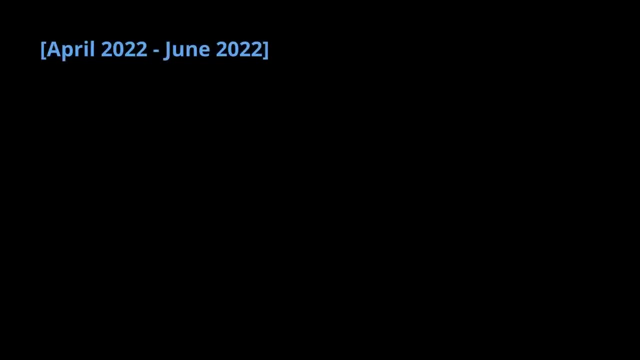 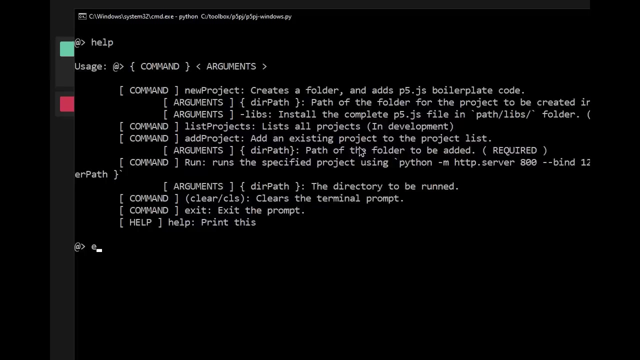 were largely hyperbole, though More on this later. At this time I felt like C was a fun language to use, but my next project was in Java. for the sake of being cross platform, I made this app installation tool in 4 days in Java. Why am I bringing up Java in a video? 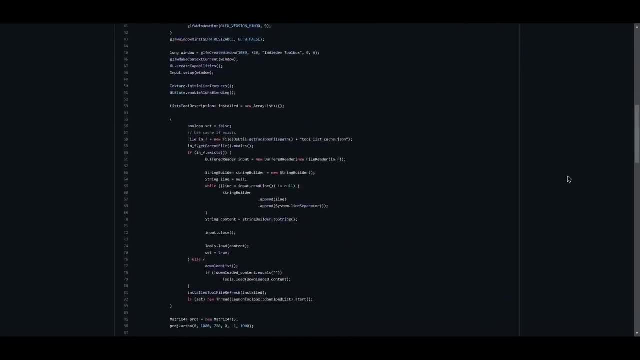 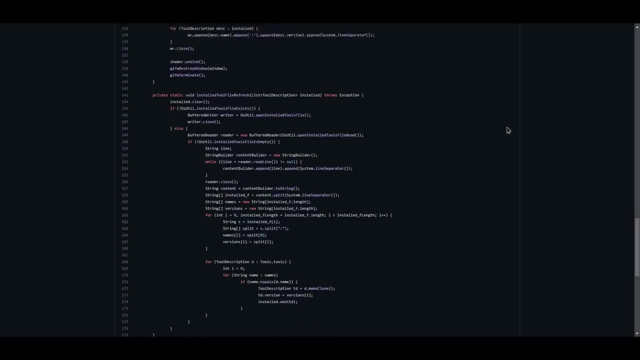 about C. Well, the whole project was written in a C star, Minimum use of classes. Any Java programmer would be shaking their fists in the air at this code, but this had led me to a big revelation. You see, when I was programming in Java, I really wasn't able to get stuff done fast at all. 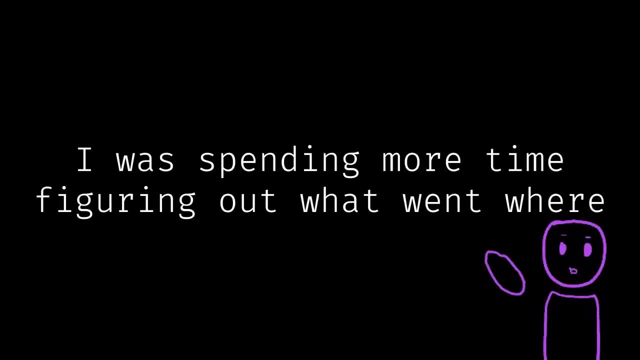 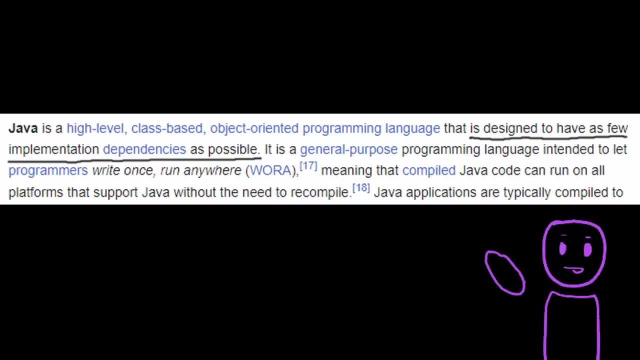 I would spend some time thinking of the best way to lay out the program structure before writing the basic code for it. It's kind of paradoxical in a way, because Java, a language with so many features ready to go, had me writing code slower than C, which is notorious. 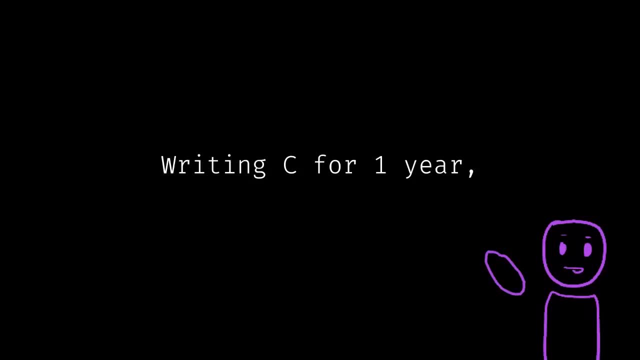 for giving you literally nothing to work with. So, with writing C for one year, then switching back to Java with the C mindset, really allowed me to finish something fast. I was studying chemistry, more specifically the chapter on solid state geometry. That's when I figured. 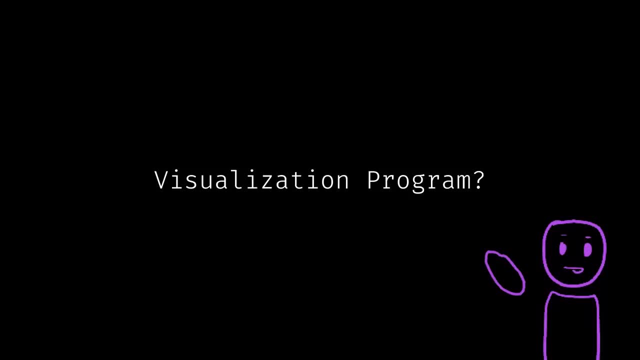 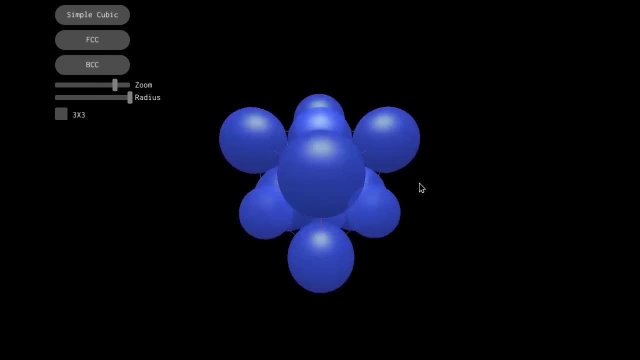 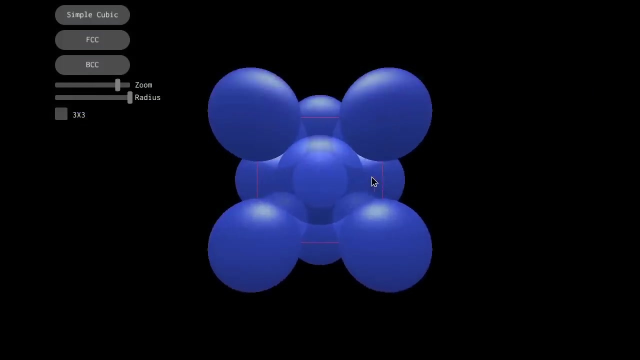 since I was projectless at the time, why not make a visualization program for this? So in about 2 weeks I made this. It's a 3D solid state geometry viewer and the first project in which I set up a crude base layer with stuff like strings and memory, allocators and generic 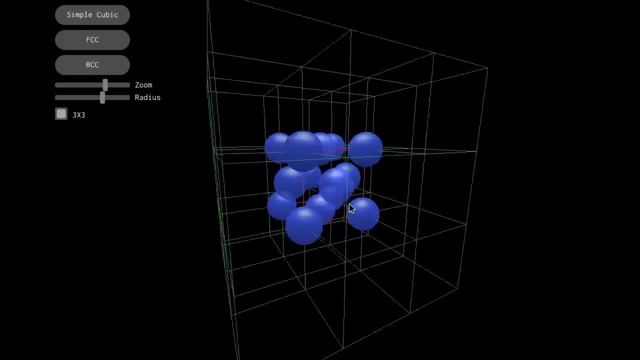 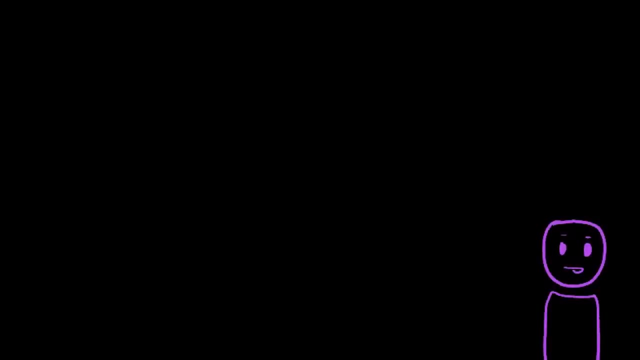 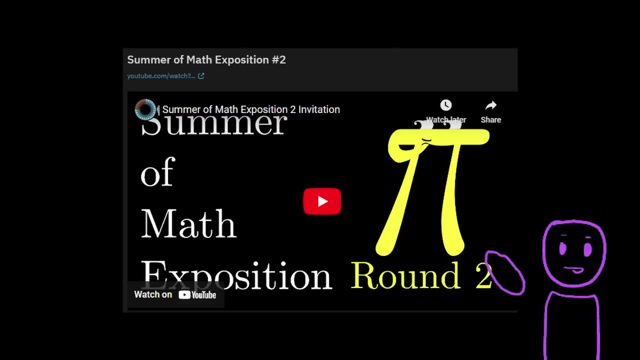 data structures and other things. This was also my first finished 3D project ever, so that was nice. Next up was another non-C project. Me and my friend took part in 3Blue1brand's SUM2 competition and made a game for it in Unity- Also a project where my old programming language 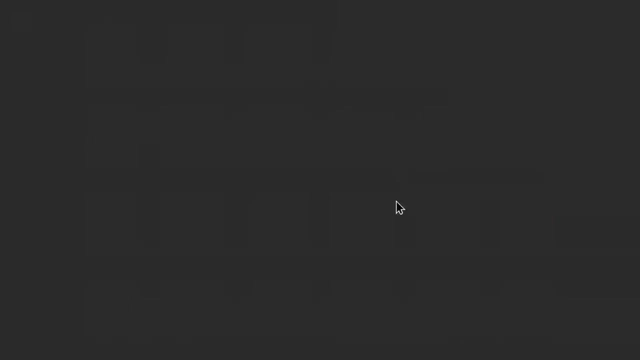 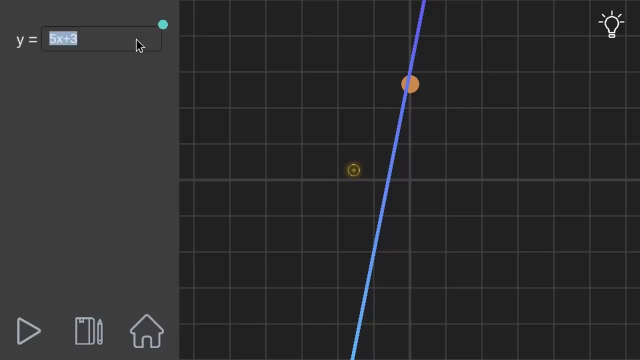 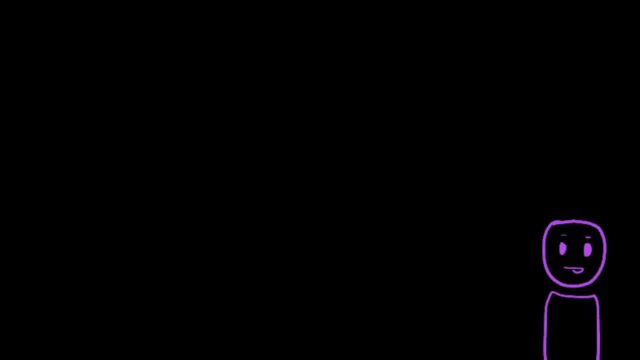 knowledge came back to help, since I had to write a math expression parser. Again, keeping the C mindset, I was really able to just do the thing, rather than beat around the bush figuring out what went where, etc. You didn't win, but getting top 100 was exciting. At the same time, I started writing a proper 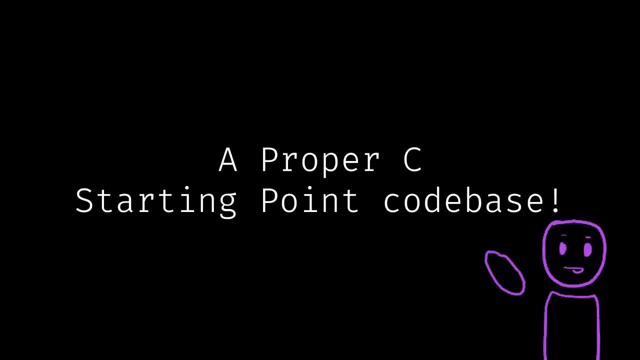 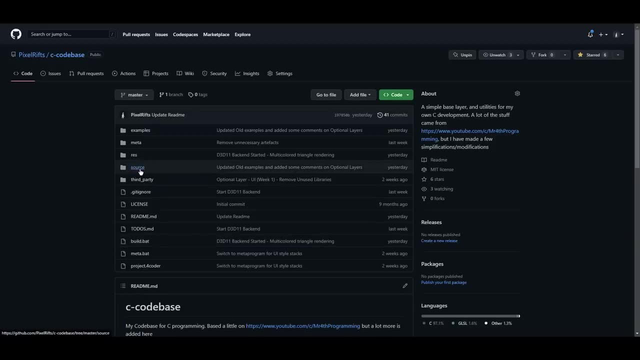 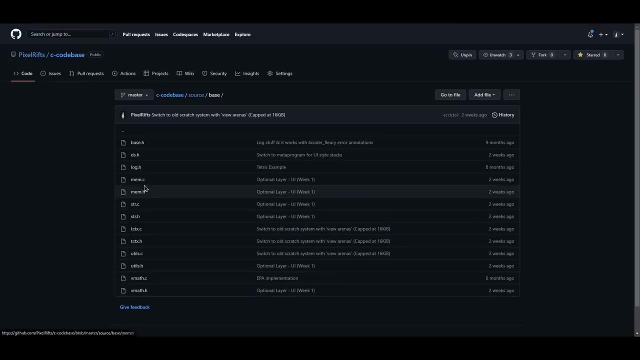 base layer in which my goal was to not use libraries at all. I also found this absolute gem of a series at that time. This base layer is one I'm working on even now, and at the time it had a lot of stuff too, For instance tried context OS specifics. 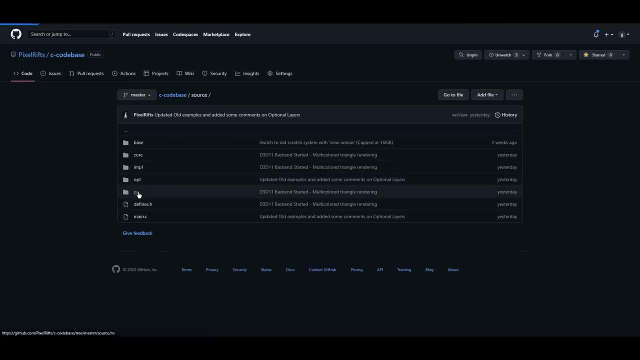 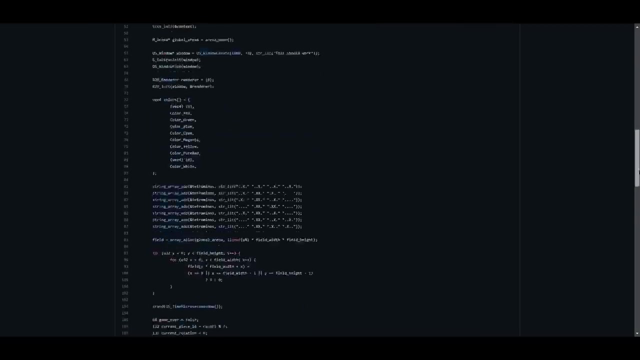 windowing OpenGL function, loading swappable backends, simple rendering utilities, generic data structures and also a small UI module that I took from the solid state visualizer I made before. I did all this without using a single library, too, Other than PNG and TTF loaders. 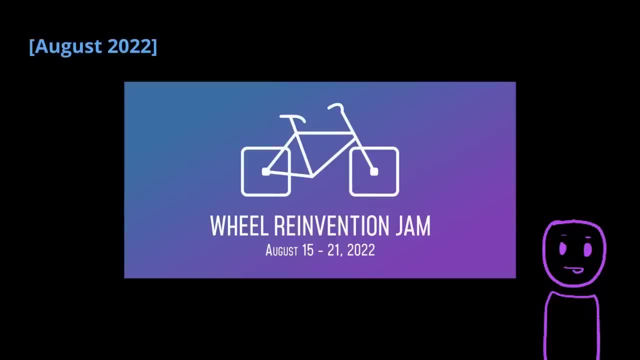 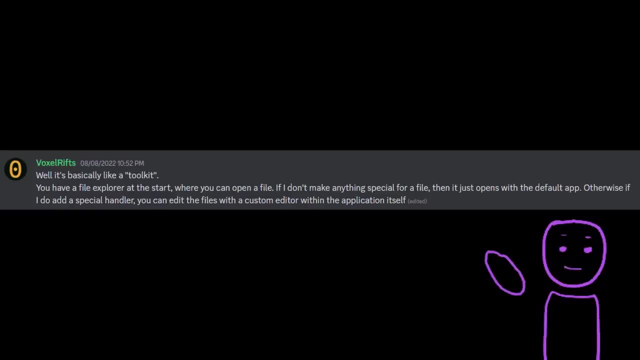 from STB, that is, It was the time of the handmade VOV invention jam. I wanted to create an application where I could create editors for any file by just adding a plugin, DLL. This was supposed to be a short project, so I spun up the prototype. 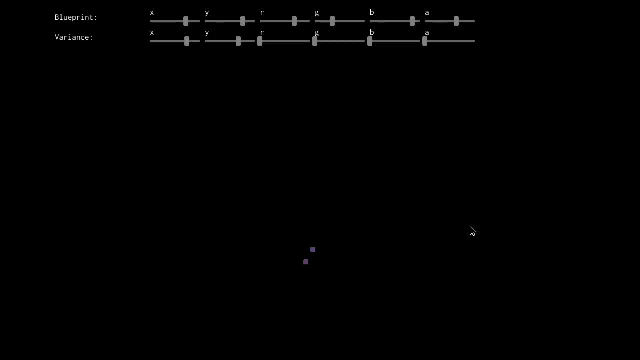 using my base layer. It had a working particle system editor and texture viewer. The base layer had made things much nicer and easier this time. I also easily embedded the solid state geometry viewer into this application. We now catch up to the present. I haven't worked. 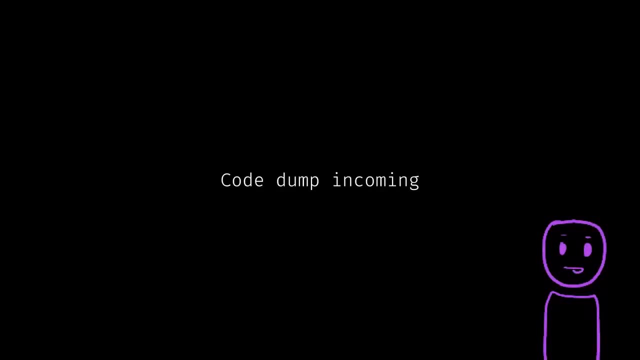 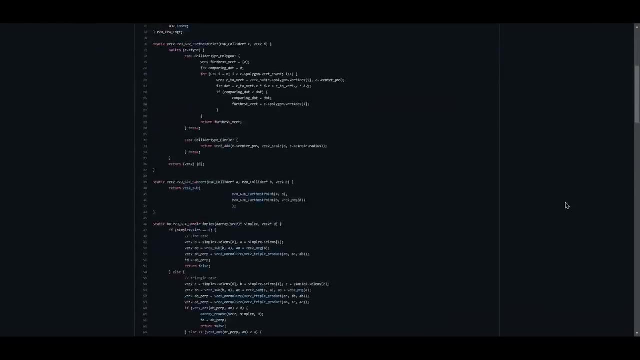 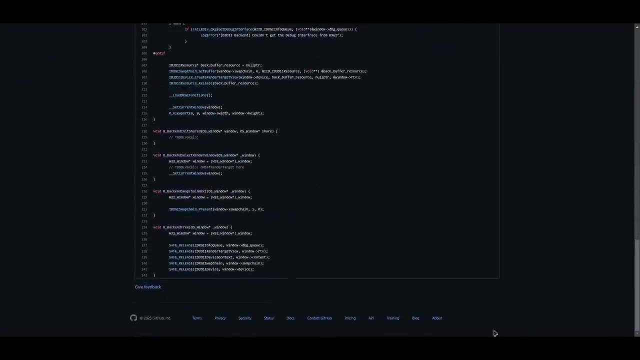 on anything major in this little while because of exams, but I still did get stuff done. I created a repo for the code base and did some miscellaneous stuff around it, like adding a collision detection and resolution, revamping the UI system, starting work on a D3D11 backend. 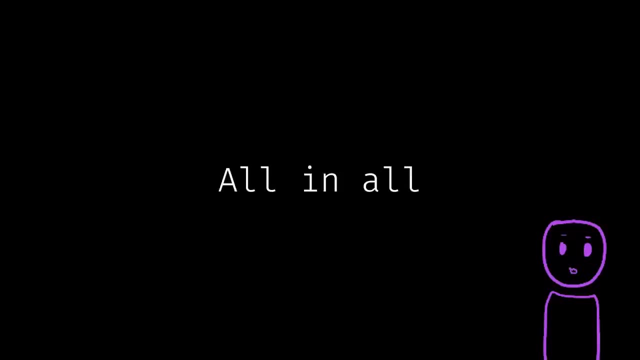 setting up metaprogramming layers and stuff like that. All in all, within the two years of C, I've gotten pretty used to it and honestly, it's one of my favorite languages by now. I also want to quickly smash some misconceptions about using C Number one, the elephant in the room- segfaults. You've probably seen memes about this. They're all hyperbole. 99% of segfaults are trivial to debug. This enables the address sanitizer or run the executable through a debugger and it'll break exactly where the access error happens. Most of the time it's because something with a null pointer and you can fix. 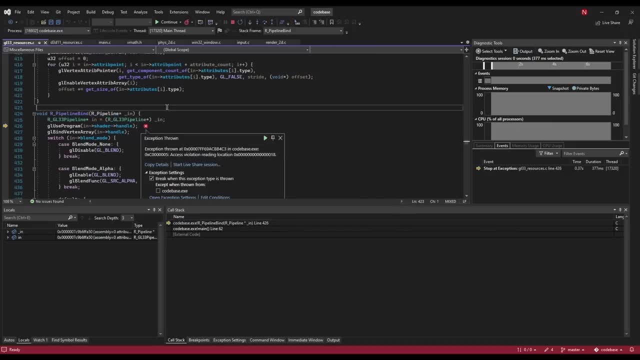 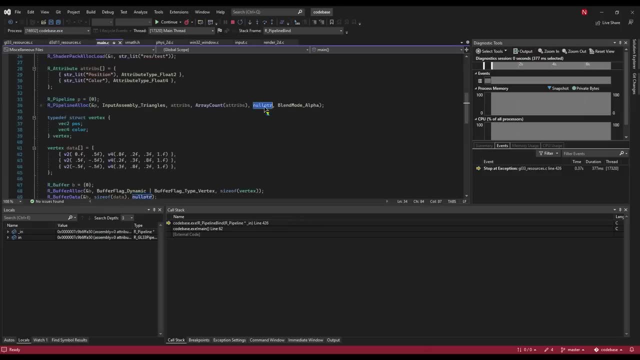 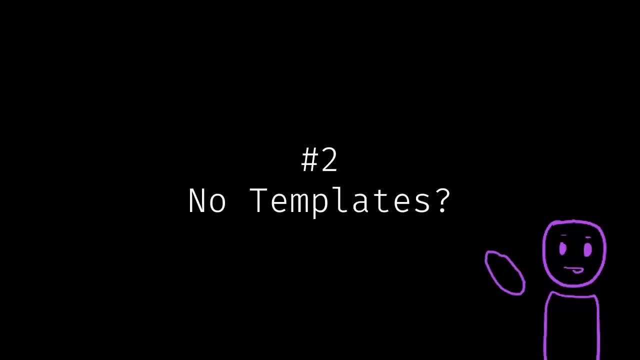 it easily. The remaining 1% are memory corruptions or overwrites, which can be caught by adding a small size tag before the allocation and making sure you're not writing beyond the given range Number two templates or the lack thereof, And I do agree this is kind of annoying. 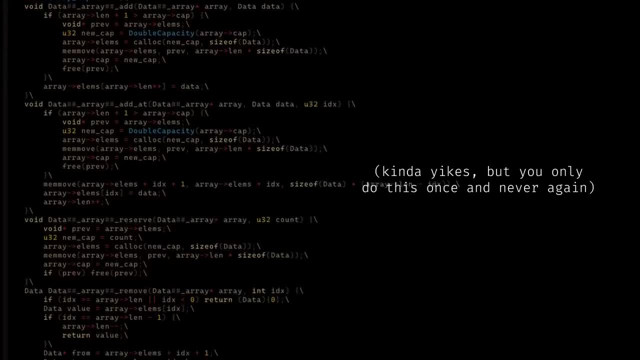 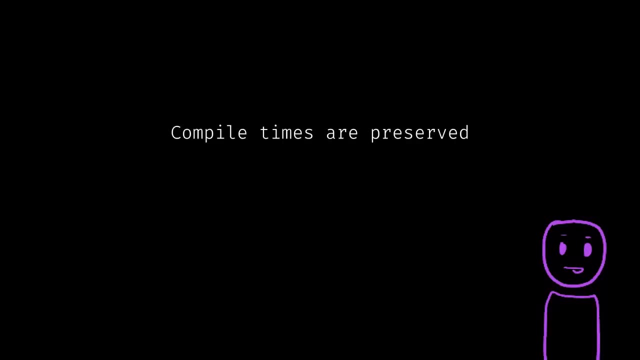 but you can get around this by implementing some macros that instantiate code for you quickly. Alternatively, you can use metaprogramming. Both of these don't really cause compile times to skyrocket and the errors aren't horrendous. The only thing is, if you're using macros, debugging errors can be somewhat tedious. 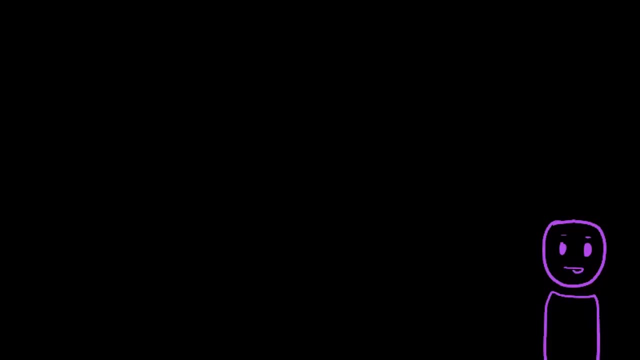 That brings us to the end of this video. If you liked this video, please leave a like, subscribe and hit the notification bell. Thank you for watching. My goal with this video was to show that some slight shift in thinking really changed my